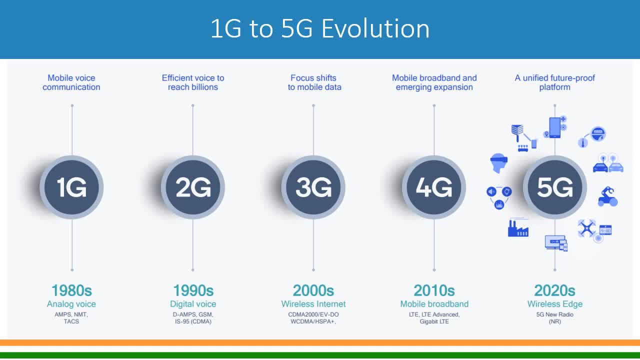 G-AMPS is a technology which is used for 2G is D-AMPS G-AMPS. G-AMPS is a technology which is used for 2G is D-AMPS G-AMPS. George Law of Second Generation technology, IS95, CDMA. 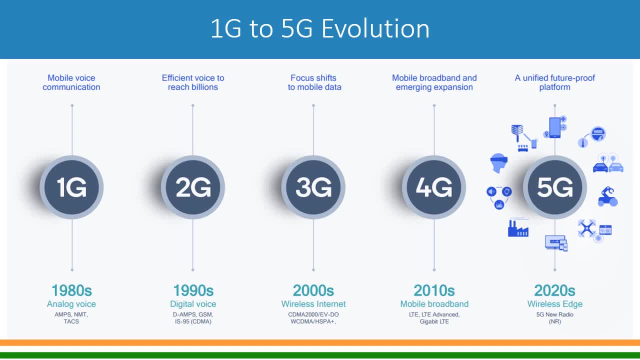 Out of these technologies, GSM has survived even today. In many country 2G services are offered using the GSM technologies. Then again from 1990s to 2000,. in a 10 years gap came the 3G and the focus shifted from voice toett. 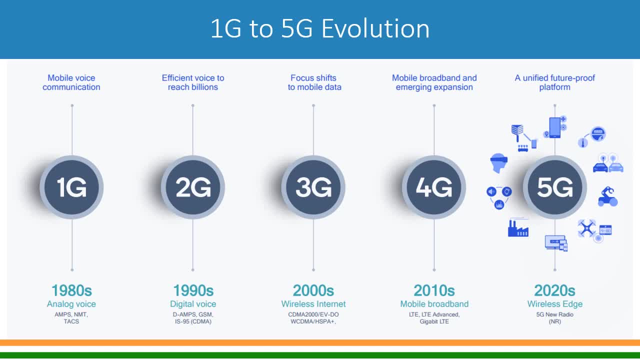 We started enjoying the wireless internet And the technologies which were approved by ITU as 3G were CDMA 2000, EVDO and WCDMA and HSPA on the GSM side, And the 3G network in India is still running by some of the operators like BSNL. Other operators have moved to the 4G services, So from 2000 to 2010,. again within the span of 10 years. 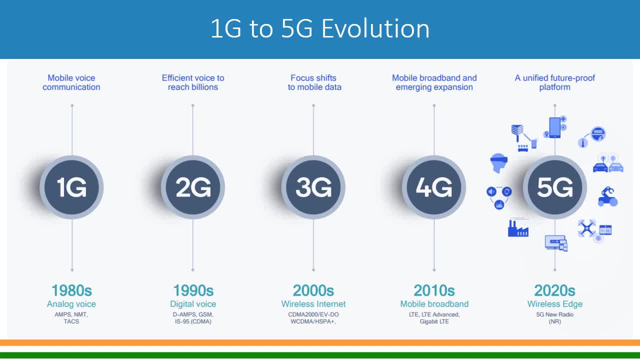 So what? we see? that every 10 years there is a jump from one generation of mobile telephony to other generation of mobile telephony. So in 2010,. 4G came, And here the focus shifted on mobile broadband, that is, high speed internet on your mobile phone itself. And the technologies which were being used, or which are being used, rather, is LTE, LTE advanced and now gigabit LTE. 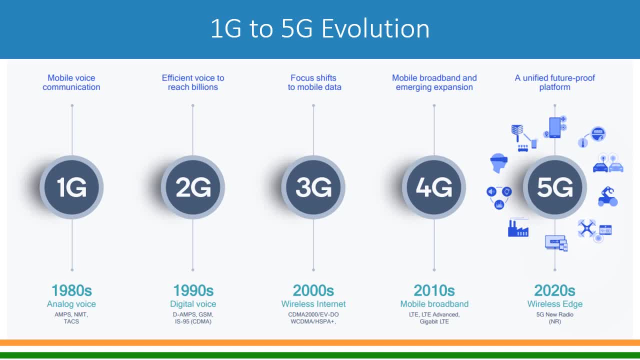 So, again, from 2010 to 2020, the focus is moving from 4G to 5G, And 5G is being said as a unified future proof platform, So this will give very, very high speed internet. You can see my video on 5G introductions, wherein I have given detail of 5G. 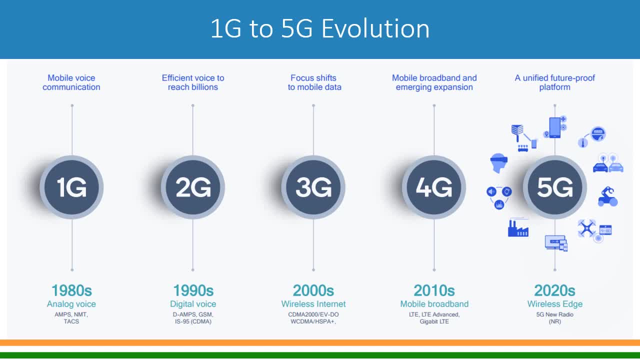 And we also see the wireless edge kind of services coming up because of the 5G architecture. So this will give very, very high speed internet. You can see my video on 5G introductions, wherein I have given detail of 5G. 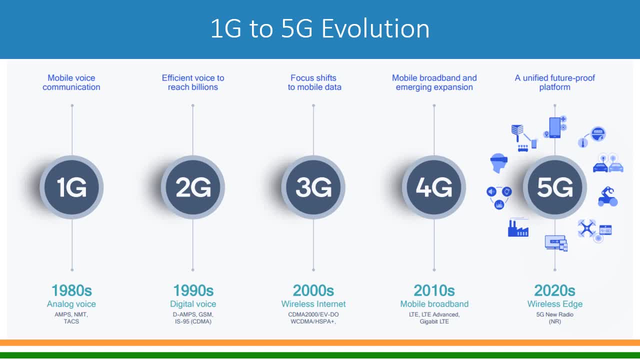 And again by 2020, the focus would be on 6G, AR, THROUGH 4G And with a variety of applications available and it has got a new. So the variety of services tell of, for example, enhanced mobile broad band, ultra-reliable. 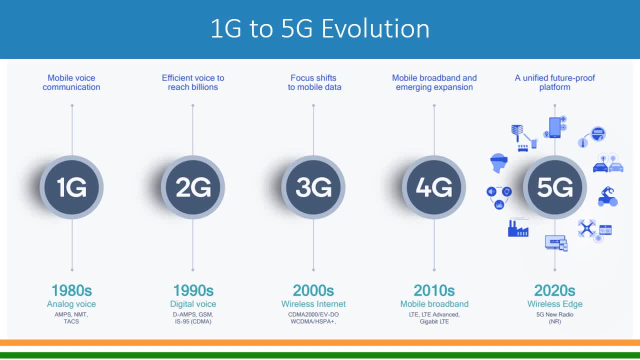 low-latency kind of services and massive machine type communication like IoT and sensors, And it operates. it can operates from sub one gigahertz frequency to millimeter wave and, using my memento, been forming kind of technologies And the technologies we have discovered over than 50 years that are actually now coming and we should breeze through this years in a whale size scale. as this can also be a very kind of new medium, and today it's changing so much, But by 2020, this is going get promised, getting kind of reimagоду κά Geongula- ground lived which is being formed from $3.5 million lux. 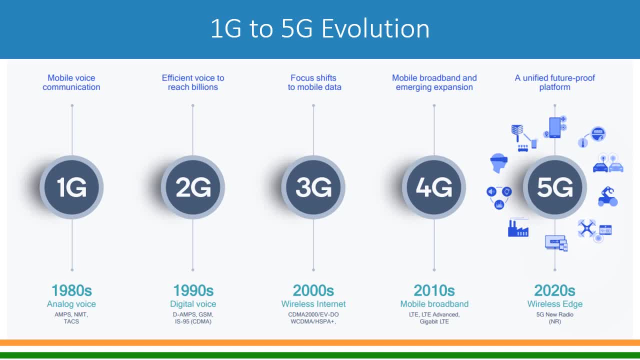 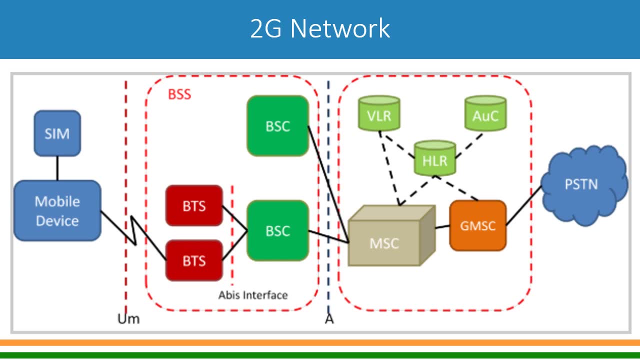 cell to achieve all these requirements. so now let us look at the network diagram of 2g second-generation mobile telecommunications. so we all know that we have a mobile device and it has got sim now on the radio part, if you see here. so you have base stations, we see towers, so base stations, antennas are. 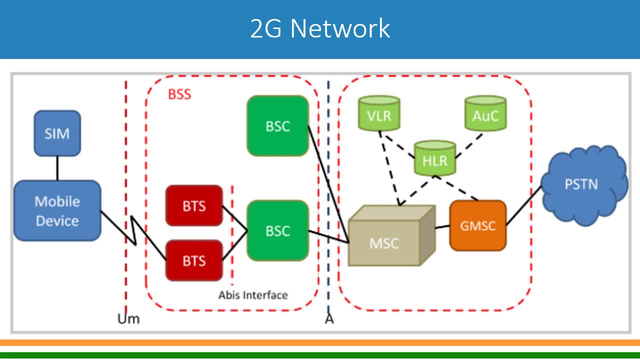 installed at tower and on the below tower you have BTS and the BTS's are connecting to base station controller, BSC, and the entire system is called BSS. and then, if you move towards core side, core network, you have MSC, mobile switching center, which connects all the BSCs. then you have GMSC, gateway MSC, which connects to 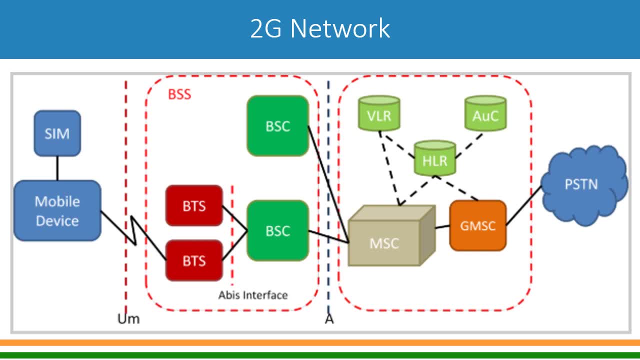 outside network like PSTN. you have HLR home location register where detail of all the subscribers are stored, and then you have VLR visitor location register. all the roaming subscribers details are kept here. so primarily 2g network is a circuit switch to network and if you see, here we have BSTN GMSC and then we have a BSTN gateway MSC which is 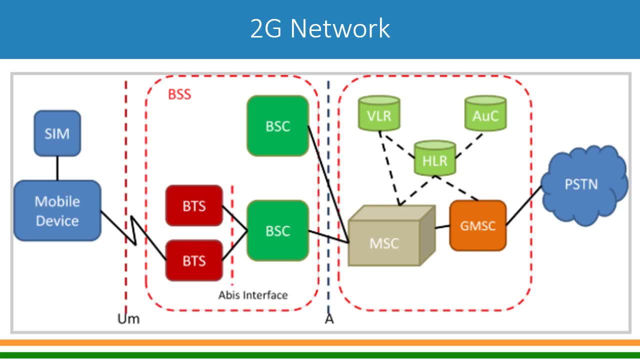 on the radio side it uses time division, multiplexing. for every mobile call there is a specific time slot allotted and that gets, I mean that allotment continues till call is continuing. so that means that is a dedicated voice channel even on the radio and of course that will continue on to the MSC and 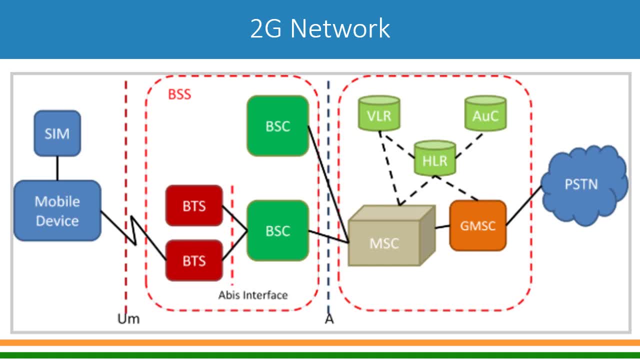 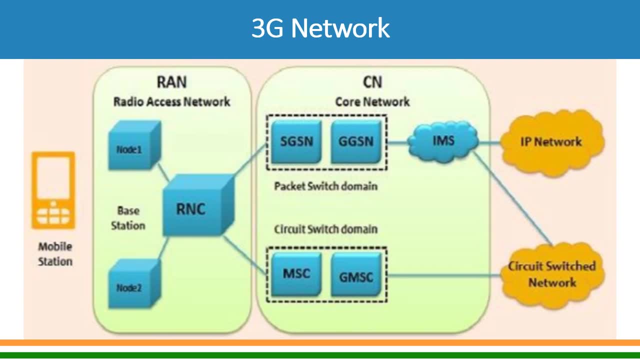 beyond. so primarily 2G is a circuit switched network. now let us look at 3G network, how it evolved from 2G to 3G. so if you look at here, it is mobile station or a mobile phone. so it is similar, same, but on the radio side. so this is called. 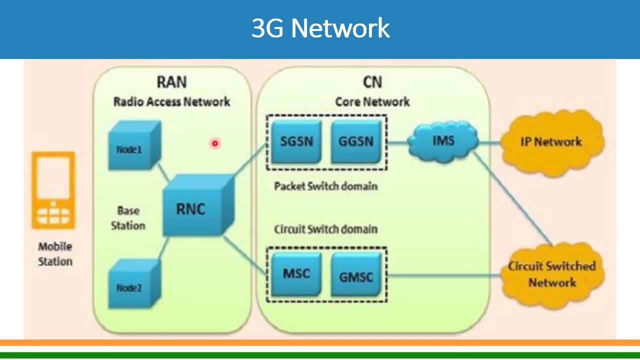 now radio access network and you have radio access network and you have radio access network and you have node node 1, node 2, so these are base node node 1, node 2, so these are base node node 1, node 2, so these are base stations. so now base stations are now. 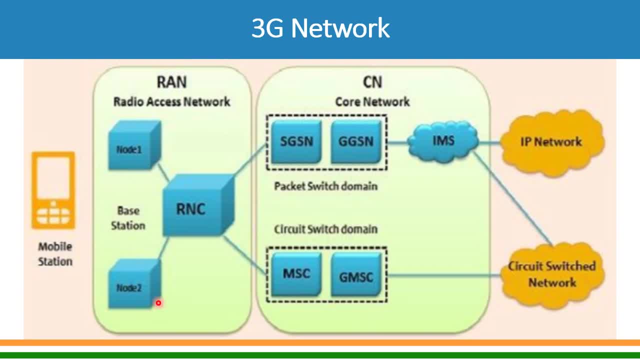 stations. so now base stations are now stations. so now base stations are now being called: node 1 in 2g, it was being being called node 1 in 2g. it was being being called node 1 in 2g, it was being called BTS and the BSC is being called. 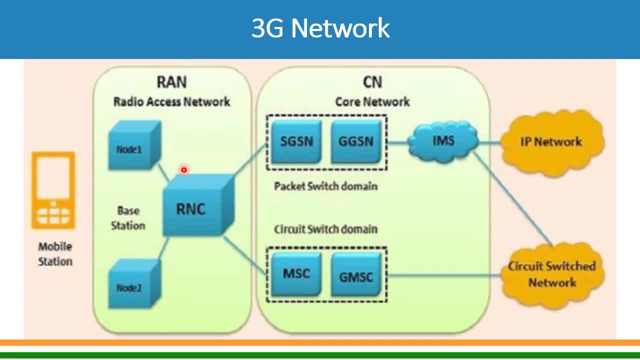 called BTS and the BSC is being called called BTS and the BSC is being called as a radio network controller. some names as a radio network controller. some names as a radio network controller. some names have changed, but this is equivalent to have changed, but this is equivalent to. 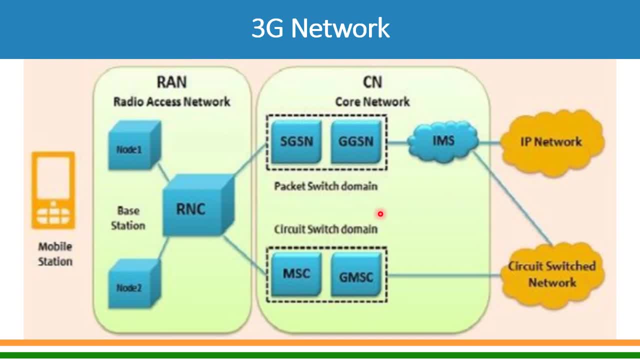 have changed, but this is equivalent to BSC on the core side. there is a BSC on the core side. there is a BSC on the core side. there is a difference. so the core is having two difference. so the core is having two difference. so the core is having two parts. one is a circuit switch domain. 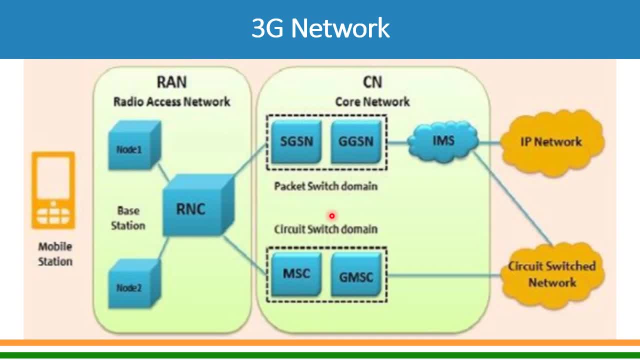 parts one is a circuit switch domain. parts one is a circuit switch domain which is similar or same to the 2g, which is similar or same to the 2g, which is similar or same to the 2g network. in addition, a packet code network. in addition, a packet code. 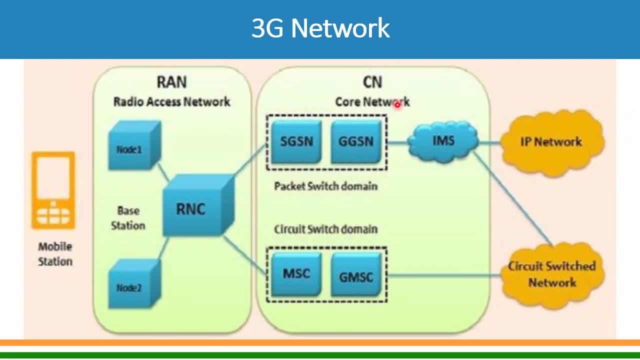 network. in addition, a packet code network has been introduced. so that is network has been introduced. so that is, network has been introduced. so that is packet switch domain. so now all the packet switch domain. so now all the packet switch domain. so now all the voice call will continue to be handled on. 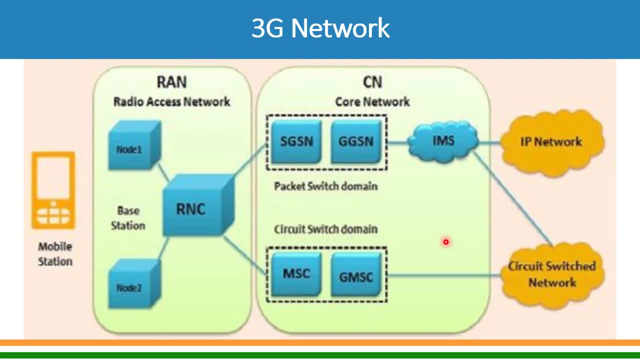 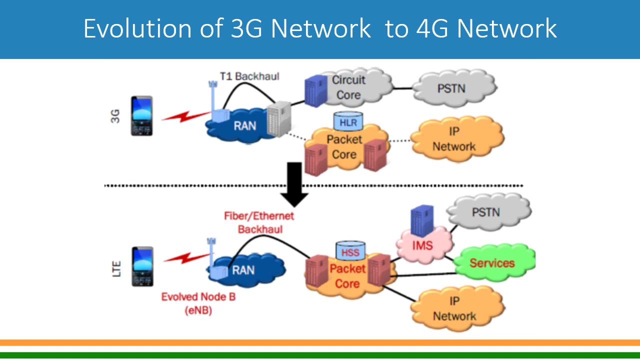 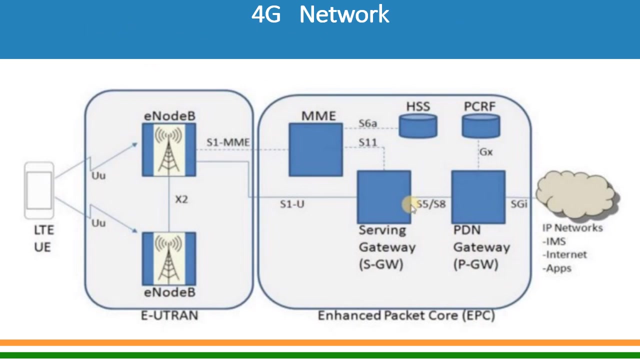 voice call will continue to be handled on. voice call will continue to be handled on the circuit switch domain. but all the the circuit switch domain, but all the the circuit switch domain, but all the data, data, data, various, various, various. network element like MME- this is. network element like MME- this is. 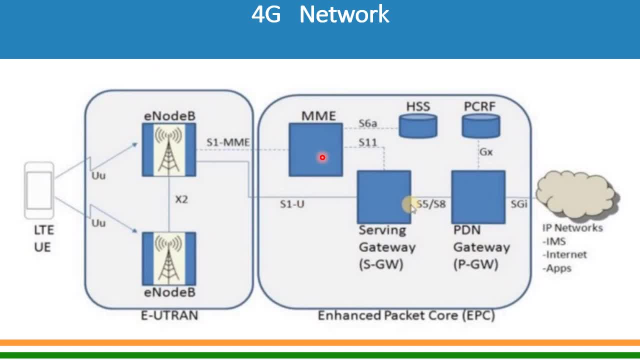 network element, like MME. this is mobility management entity, which is mobility management entity, which is mobility management entity, which is responsible for mobility management, responsible for mobility management, responsible for mobility management, session management, and also it connects session management and also it connects session management and also it connects UE for NAS signaling. it also does some. 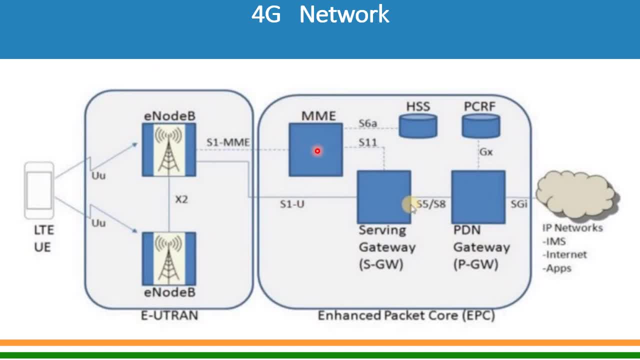 UE for NAS signaling. it also does some UE for NAS signaling. it also does some connection management, the other connection management, the other connection management, the other management, etc. on the user plane side management, etc. on the user plane side management, etc. on the user plane side data traffic flows so the data traffic will. 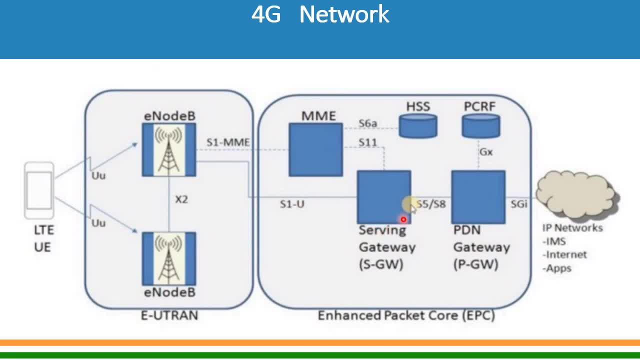 data traffic flows, so the data traffic will. data traffic flows, so the data traffic will flow from UE to eNodeB to serving flow from UE to eNodeB, to serving flow from UE to eNodeB. to serving gateway to PDN, gateway to the IP. 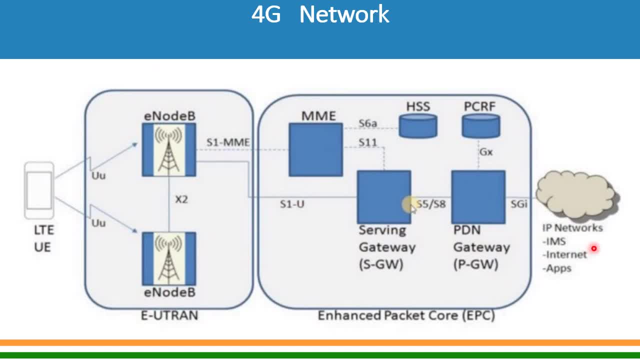 gateway to PDN, gateway to the IP gateway to PDN, gateway to the IP network or any other network like IMS network or any other network like IMS network or any other network like IMS internet or any apps. so so user plane, internet or any apps, so so user plane. 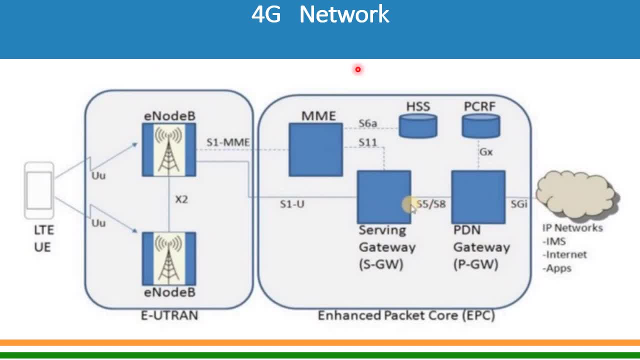 internet or any apps. so so user plane goes like this user plane, data and rest goes like this. user plane, data and rest goes like this. user plane, data and rest are for managing mobility and other are for managing mobility and other are for managing mobility and other control functions. so basically the upper. 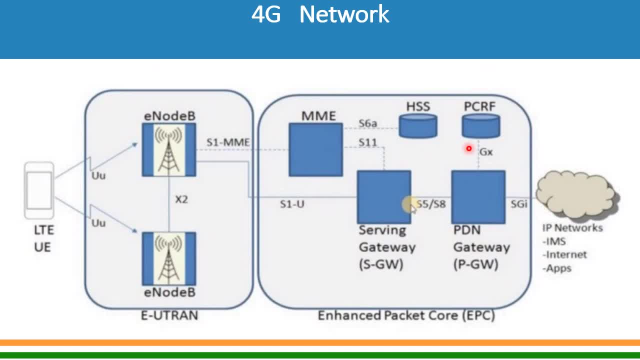 control functions, so basically the upper control functions. so basically the upper part is the pure control plane, whereas part is the pure control plane, whereas part is the pure control plane, whereas the lower part is primarily user plane. the lower part is primarily user plane. the lower part is primarily user plane, but it also does some control plane. 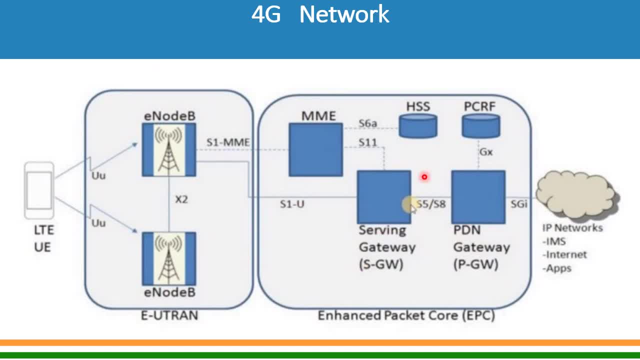 but it also does some control plane. but it also does some control plane function. so now let's look at serving function. so now let's look at serving function. so now let's look at serving gateway. so serving gateway connects to gateway. so serving gateway connects to gateway. so serving gateway connects to the eNodeB for user plane data and PDN. 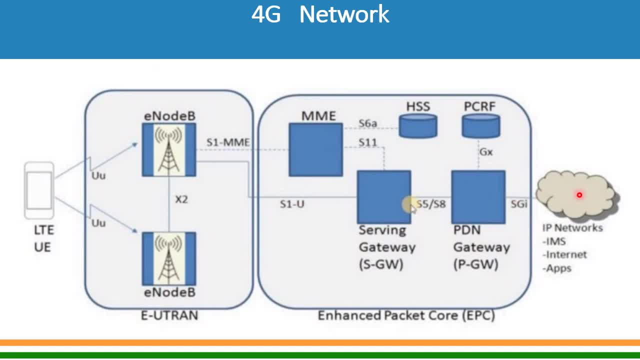 the eNodeB for user plane data and PDN. the eNodeB for user plane data and PDN gateway connects to the outside IP gateway. connects to the outside IP gateway. connects to the outside IP network on SGI interface. so all the data network on SGI interface. so all the data. 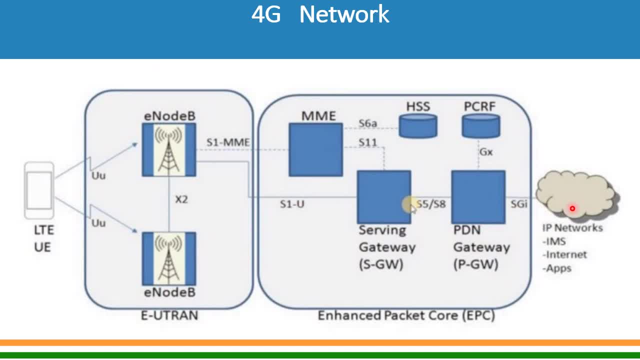 network on SGI interface. so all the data towards IP network goes through PDN, towards IP network, goes through PDN, towards IP network goes through PDN gateway. so as the name suggests, this is gateway. so as the name suggests, this is gateway. so as the name suggests, this is gateway towards IP network and serving 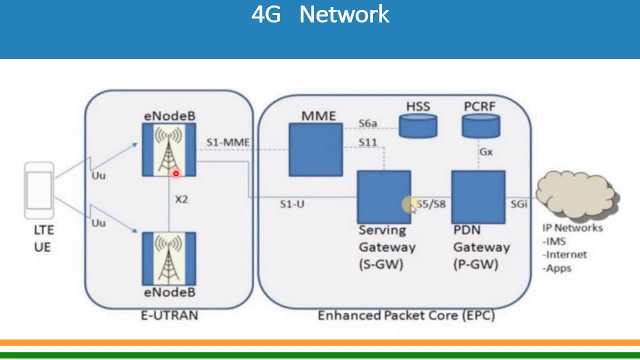 gateway towards IP network and serving gateway towards IP network and serving gateway is gateway towards eNodeB. now gateway is gateway towards eNodeB. now gateway is gateway towards eNodeB. now let us look at various interfaces which, let us look at various interfaces which, let us look at various interfaces which is used in 4G network. so the interface, 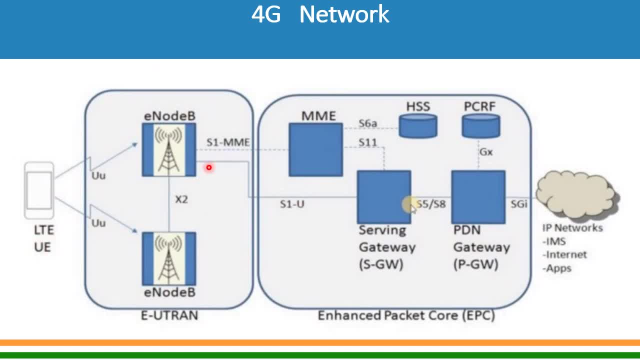 is used in 4G network, so the interface is used in 4G network. so the interface- radio interface between mobile- and the radio interface between mobile and the radio interface between mobile and the eNodeB is called UU interface and the eNodeB is called UU interface and the 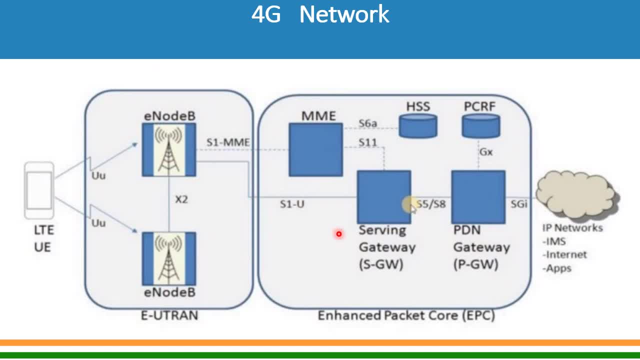 eNodeB is called UU interface and the interface user plane interface between interface user plane interface between interface user plane interface between eNodeB to serving gateway, which is eNodeB to serving gateway, which is eNodeB to serving gateway, which is primarily for data traffic. the actual 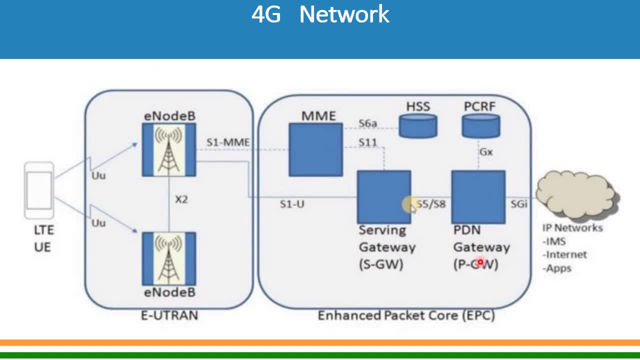 primarily for data traffic, the actual, primarily for data traffic, the actual data traffic flows here. so that is called data traffic flows here. so that is called data traffic flows here. so that is called S1U, and then you have interface: S1U, and then you have interface. 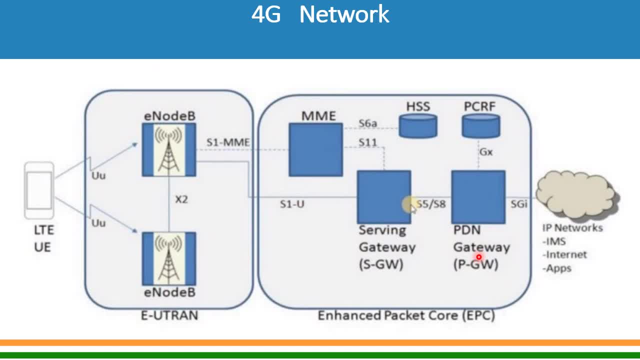 S1U, and then you have interface between serving gateway and PDN gateway, between serving gateway and PDN gateway, between serving gateway and PDN gateway- S5 or asset- and then you have SDI S5 or asset, and then you have SDI S5 or asset and then you have SDI interface to IP network from PDN. so if 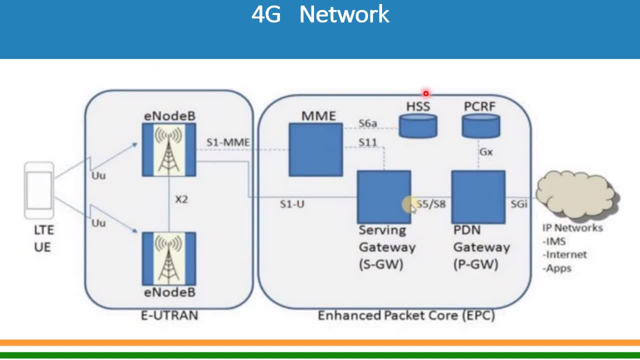 interface to IP network from PDN. so if interface to IP network from PDN. so if you look at HSS- we had discussed that. you look at HSS. we had discussed that. you look at HSS. we had discussed that this is home subscribers server. so all. 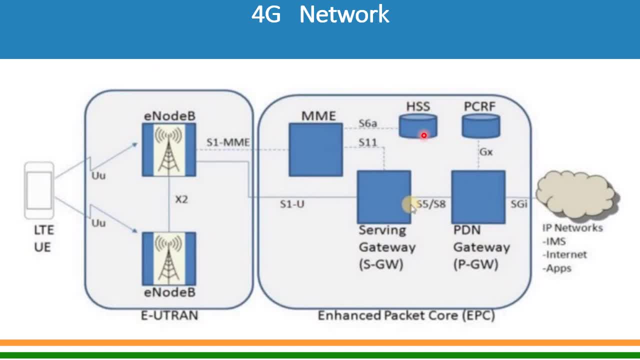 this is home subscribers server, so all this is home subscribers server, so all the subscriber informations are kept. the subscriber informations are kept. the subscriber informations are kept here and we have PCRF policy charging here and we have PCRF policy charging here and we have PCRF policy charging function policy and charging function. so 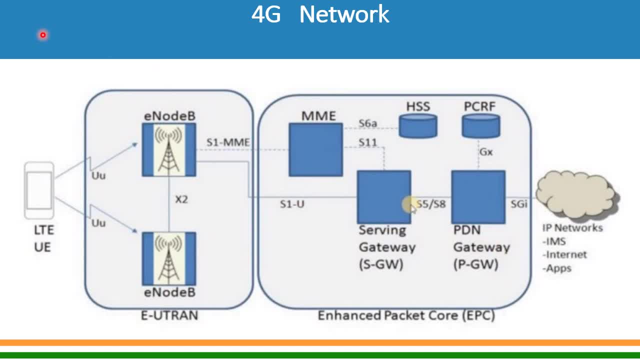 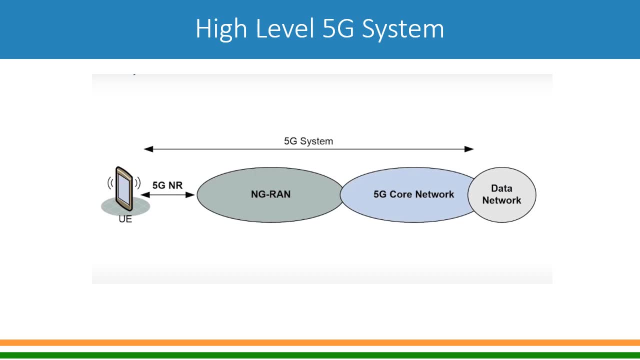 function policy and charging function. so function policy and charging function. so this is how a 4G network. this is how a 4G network. this is how a 4G network looks like. now let us look at high level 5g system. so you have ue user equipment, that is, mobile 5g. 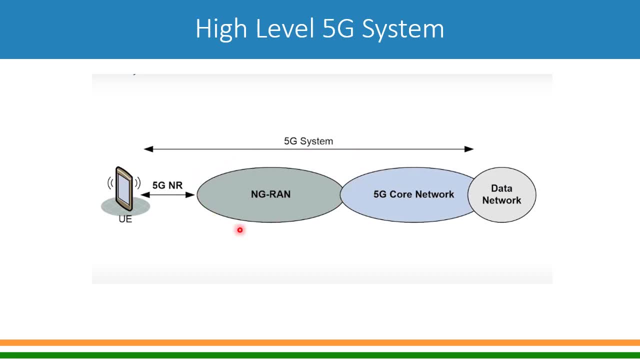 mobile and the radio part is called ng ram, new generation radio access network. and then you have code, so that is called 5g code and then it connects to data network. so so in 4g this was being called packet data network, where in 5g it is just called data network. but because it can, 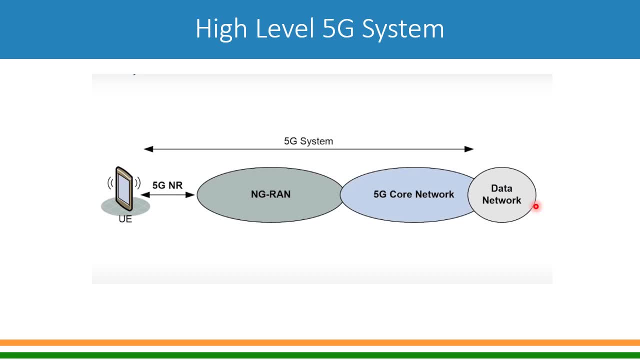 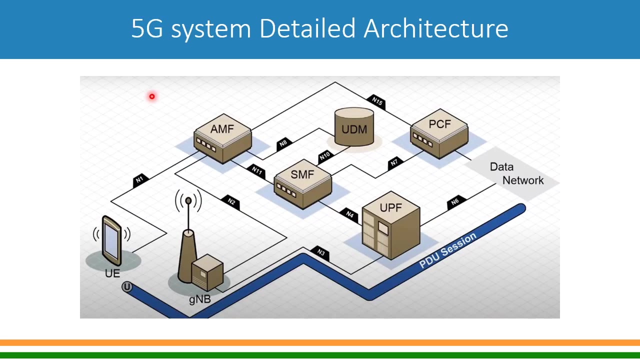 have any kind of data network, not only the packet data network, even the structured data is supported in 5g, so the entire thing is called 5g system. so let us look at 5g system in slightly detailed architecture. so you have ue and then you have g, node b. that is your node b. 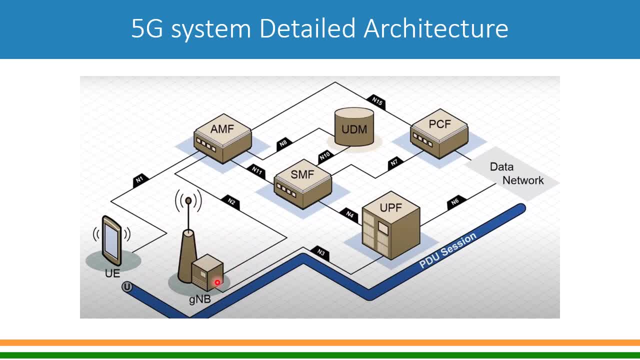 e, e node b in 4g, here it is called g node b, and then you have user plane function and then you have data network. so the actual data traffic from mobile to a data network will be flowing from ue to g node b to user plane function. 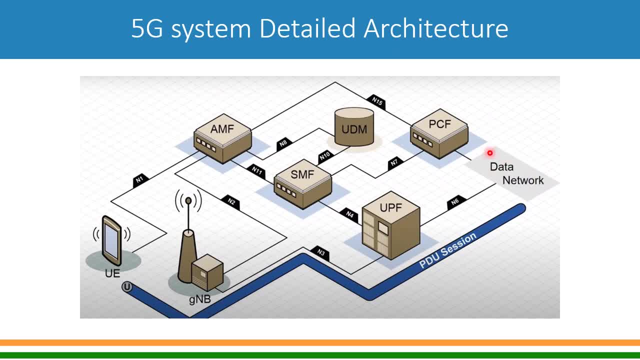 to the data network and rest. all are to support this traffic flow. so let us discuss one by one. what are these different network elements in very brief? so you have amf, that is, access and mobility functions. this is called core access and mobility function. so the ue also gets connected to amf on n1 interface, of course, through g node b. 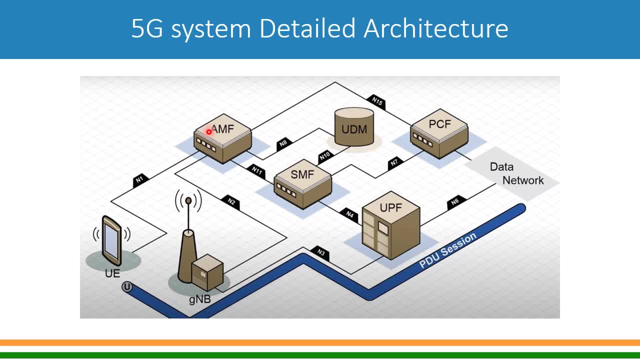 so, although interface is shown directly, but it is through g node b, only g node b transparently passes this interface to amf. so all the access authorization and mobility management is done by amf. now let us talk about smf. this is session management function. so as 5d is a pure data network, i mean the entire traffic is. 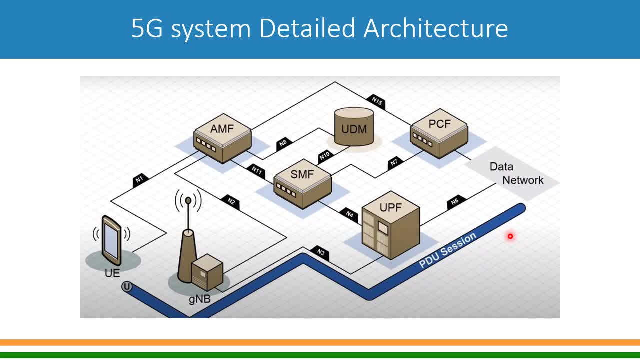 data, whether it is voice or internet or any kind of services on data. so the creation of session or modification of session or altering obsession is done by smf and this is called pdu session protocol. data unit session is established by sms for ue to make data traffic or the traffic, any kind of traffic, it has. 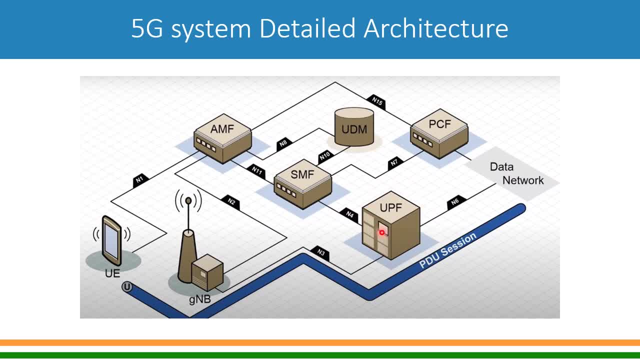 and of course user plane functions enables the ue for this data flow. and user plane function is kind of an anchor point for ue when it moves from one g node p to other g node p. cause every other data doc has attention. let us talk about udm now. let us talk about udm. 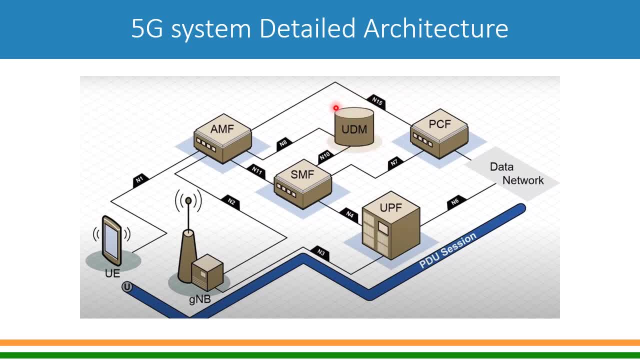 this is called unified data management. this is almost equivalent to. now let us talk about udm. this is called unified data management. this is almost equivalent to. So there could be many type of data network connected for different services. So this will also have profile of data network and which data network can be assigned to. 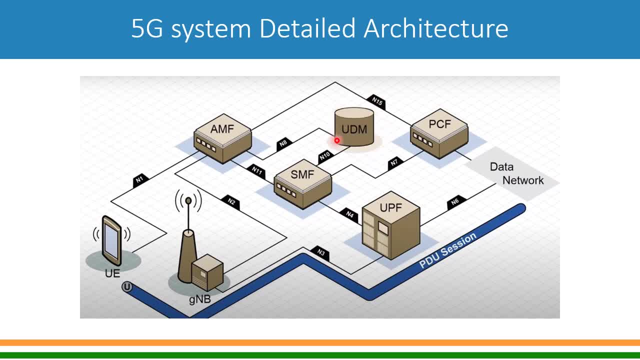 which user is also written here. and UDM also does some security related function, like if subscriber is to be authenticated. so all those security mechanism is done by UDM. Of course you have authentication function also, which is not shown here, and then you have policy and charging function- PCF for all policy and charging rules is provided. 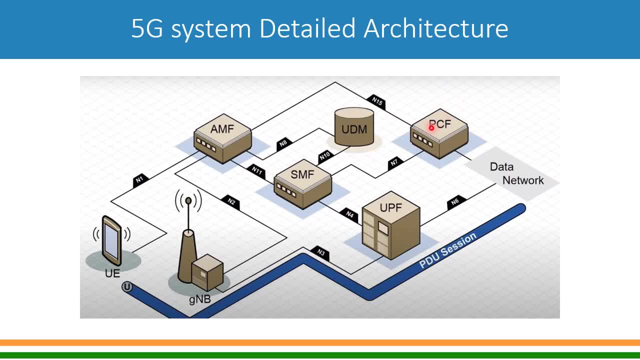 by PCF. So this is, in that cell, a 5G architecture, And this is called reference point architectures. there is one more architecture which will actually be used in 5G, or actually being used in 5G, that I will just be discussing. 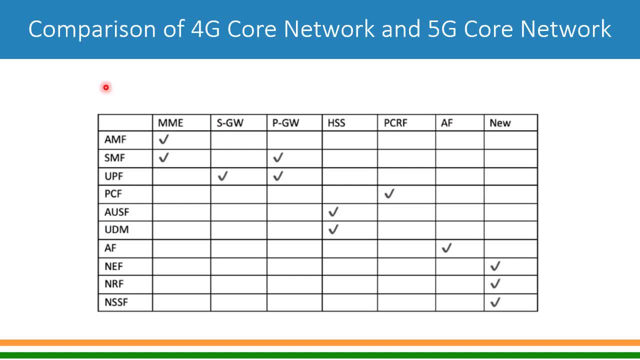 So before I move to 5G service based architecture, I just wanted to compare the 4G core network with 5G core network and which network is equivalent to which. So, for example, MME in 4G- mobility management entity in 4G- is now broken into two parts. 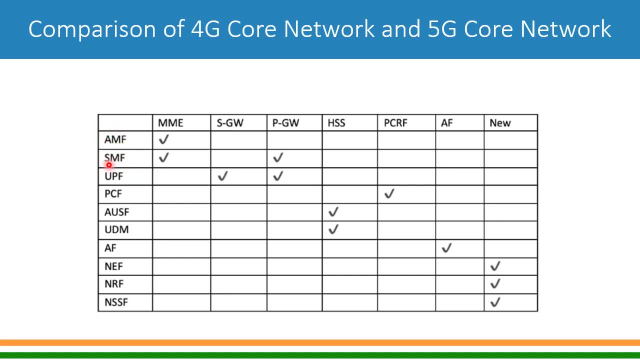 access and mobility function and session management functions. So both these functions were being done by MME in 4G network. Now user plane function in 5G has taken user plane part of the function from serving gateway and from PDN gateway. 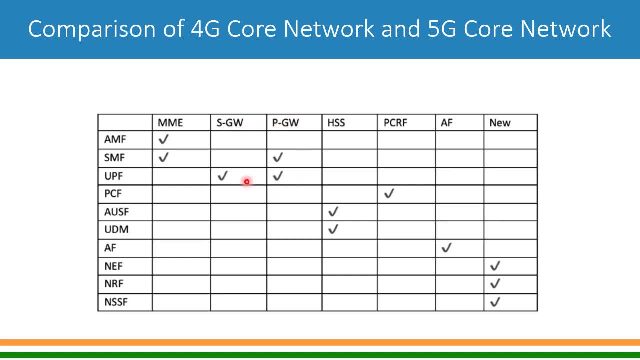 So that means serving gateway and PDN gateway is merged into UPF but only the user plane part. control plane part are not merged into the UPF. Policy and control function in 5G is equivalent to PCRF policy, control policy and charging. 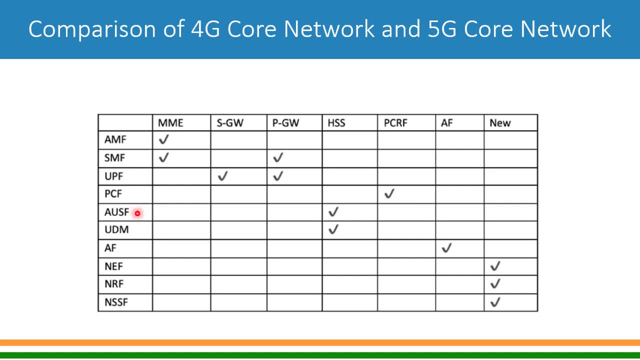 rule function in 4G And, of course, authentication function was there. So HSS was also doing authentication in case of 4G, which is now being done by AUSF, which we will discuss in the service based architecture. 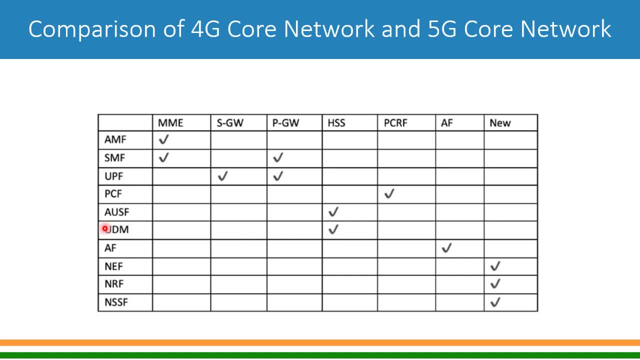 And part of the HSS function is also in the UDM- unified data management. Now, if you look at application function, it was there in the 4G, although had not shown in the simplified diagram, But application functions are there. And then in service based architecture you have some network element called network exposure. 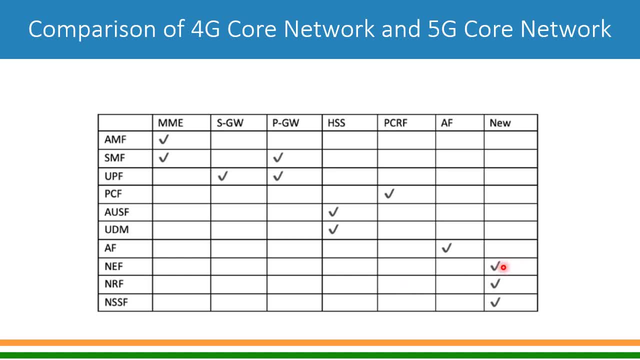 function which is a new in 5G. This is used to connect any third party system on API to 5G network, And NRF is network repository function. this is also a new element. So, since it is a service based architecture and API based, interaction will happen between 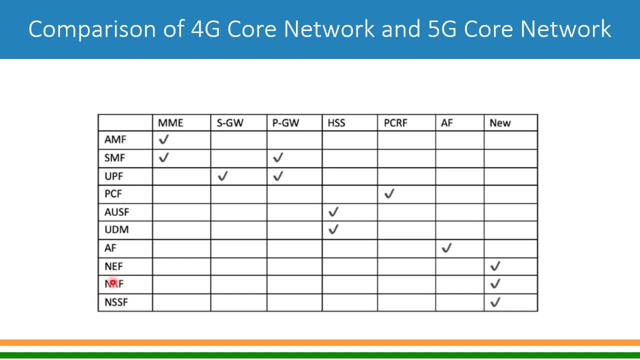 the node. So The discovery of the node will be done by NRF. And then you have very important network element called an SSF network slice selection function, which is also new. So the 5G network can be broken into various slices to offer various kinds of services. 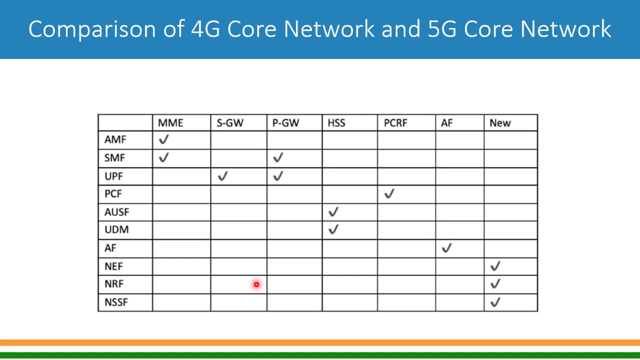 For example for enhanced mobile broadband, will have a separate slice, So it will have a different quality of service requirement: the ultra reliable, low latency kind of services like autonomous car, cell phone Or the remote surgery by a doctor. we can have a separate slice of the network which 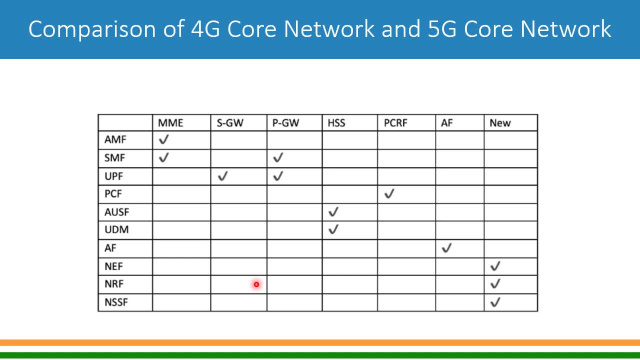 will handle this ultra reliable and low latency kind of services. Similarly, there will be a slice for sensors etc That we call it massive mobile type communication And there could be any number of slices for different purposes. There could be a slice for a specific corporate. also, one can create and allocate. 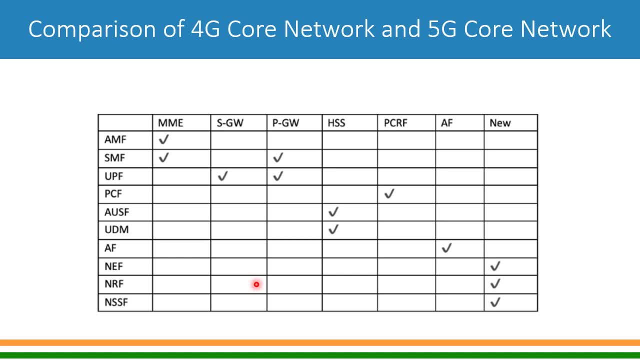 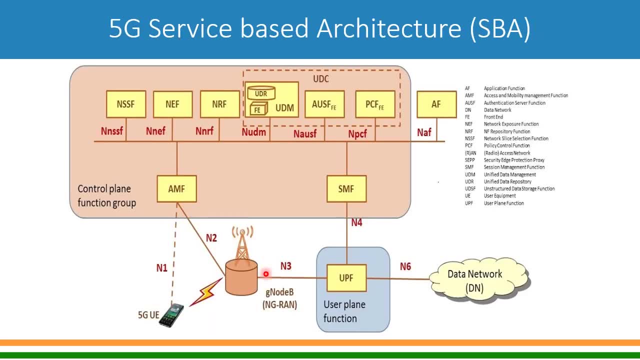 So this is a very important part. So this is a very important part. So this is a concept of slicing the end to end network of 5G. And now, finally, let us look at 5G service based architecture. So what has happened? from a point to point architecture, we have moved to a service based 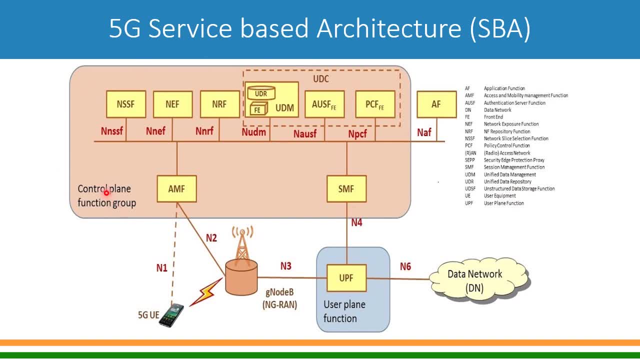 architecture. So, if you see this, this is the control plane function group And all the network element. network functions in this are connected onto a bus and they talk to each other. But you can see this looks like if you swap the user plane or consistent from API and 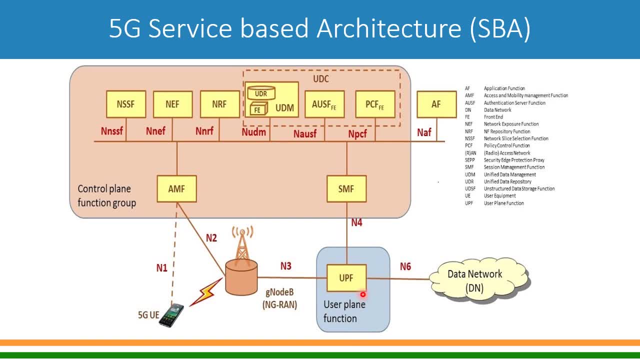 the user plane is separated out, completely separated out, and the user plane function will normally decide near to the traffic or residence itself. So it is a kind of distributed EU PF will. so the core can be centralized, but user plane function will be distributed across the network. 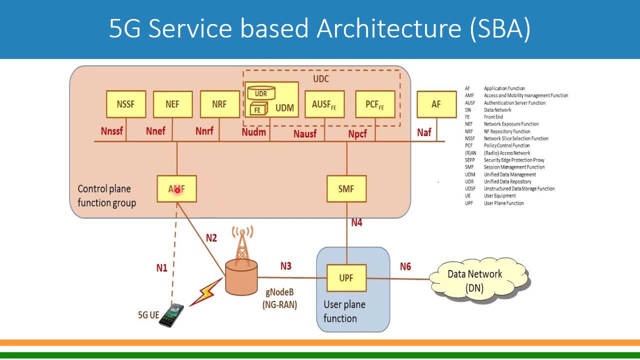 Okay, So it's very important, Wonderful. I have explained session management function. I have explained user plane functions. we have seen gNodeB mobile and how it connects to the data network. so let me just tell you the new network element. so, as I have explained, 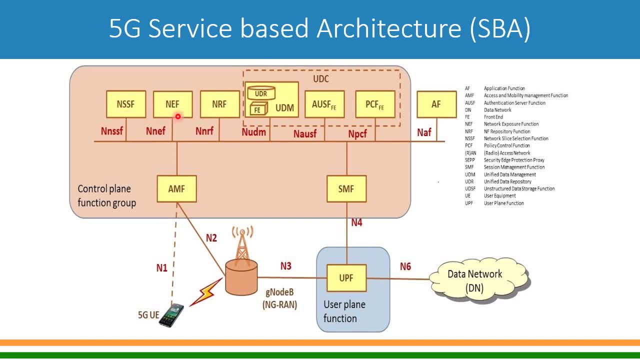 this is network slice selection functions. network exposure function for exposing the API to outside third party to connect to the 5G network. network repository functions. discovery of all the node is done by this. so suppose one network element talk to the network element, so it discovers that network. 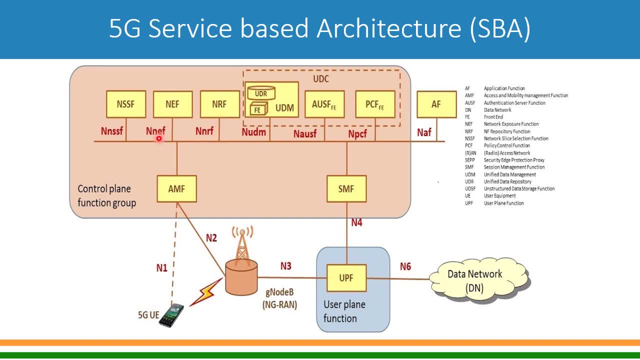 through the NRF. so if I suppose new instance of any network element is created, so NRF will have address of that, so other network element can just ping to NRF and discover that network and then they can make an API call. so it has become a flat architecture and 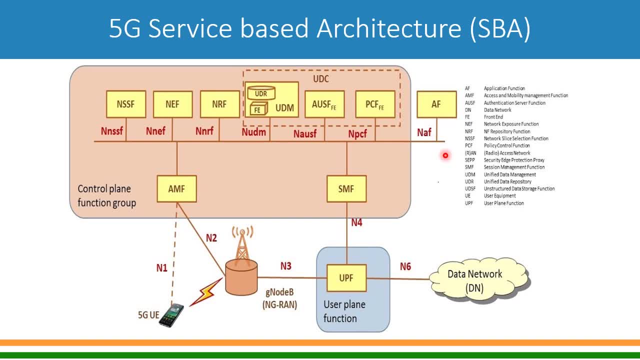 this is AF. application function has been kept outside this. this could be IMS, this could be any edge type of application and all. let us look at the user plane sites on user plane side, all the data traffic flows from UE to gNodeB to user plane function and then to the data network of any description and the 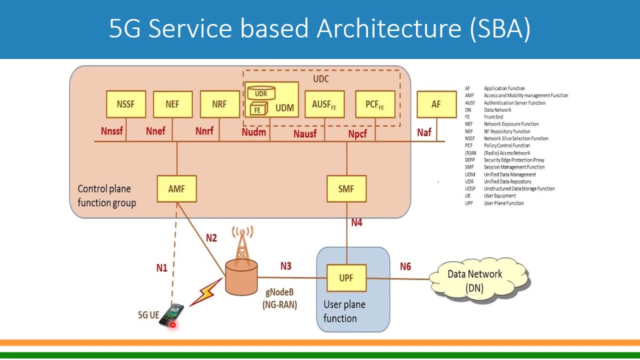 interfaces. if you look at so, interface from mobile to gNodeB, it talks to AMA form n1 interface, of course, through this and gNodeB talks to MF, on into interface. gNodeB to UPF is called and three interface and UPF two and six is. 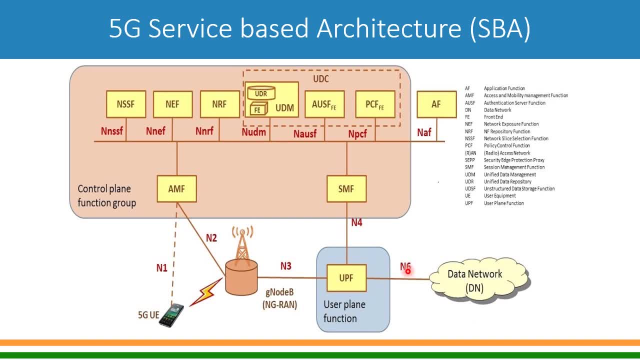 called you P of two. data network interface is an six. so on n6 interface, data network gets connected and to SMF, UPF is connected. on n4 interface and on the control panel there is no point-to-point interface. it is API based interface. so this is what I wanted to discuss with you and I have made a 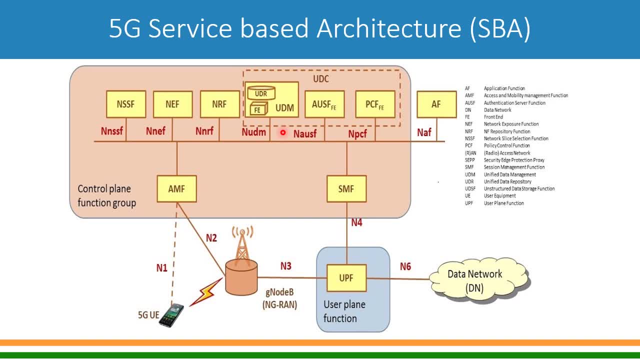 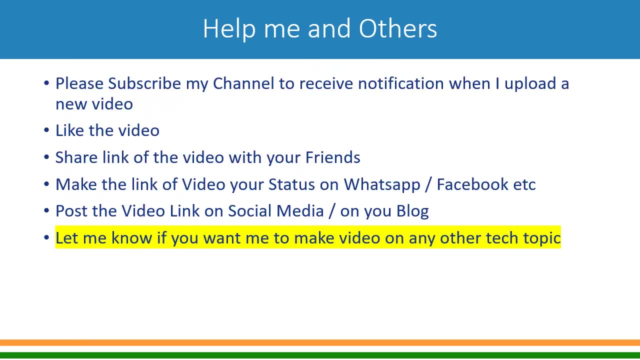 detailed presentation on the core network, we can. you can see my video in the channel if you want to go more detail on to the 5g network architecture. so thank you for listening to seeing my video on 1g to 5g: evolution of mobile. 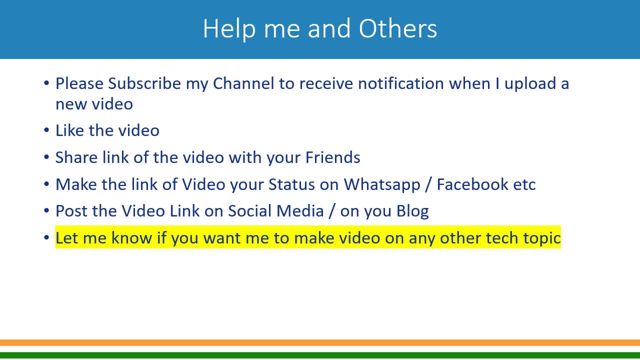 telecommunications. so please help me and help others by subscribing my channel. so if you subscribe my channel, you get a notification whenever I upload a new video on any topic. please like the video and also share the link of the video with your friends. you can make the link of the video in the description box and. 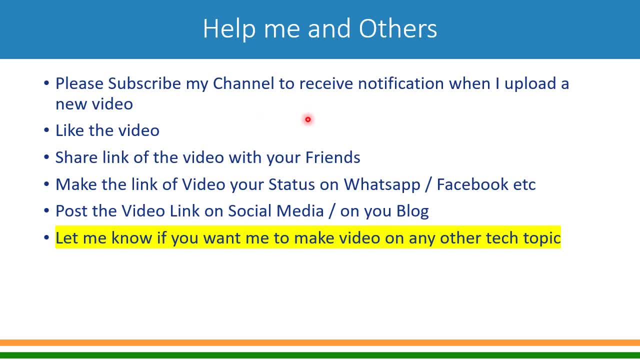 of my video as your status on whatsapp, facebook, etc. and if you use other social media, you can post video link of this particular session. if you write a blog, you can write a blog about my video and then, finally, please let me know if you want me to make video on any other topic, other tech topic, particularly on 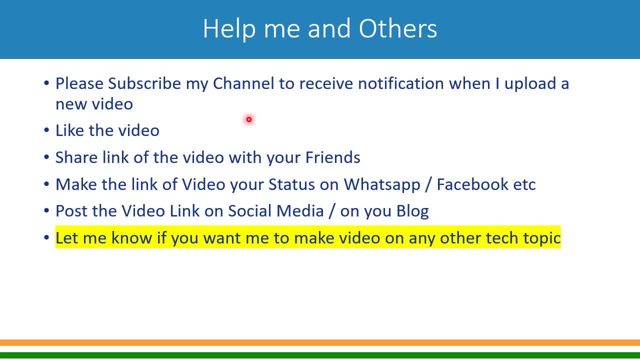 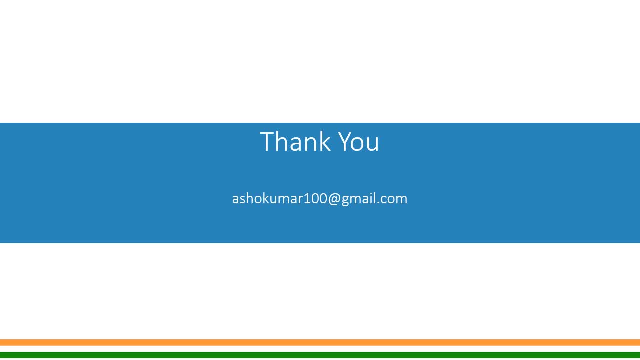 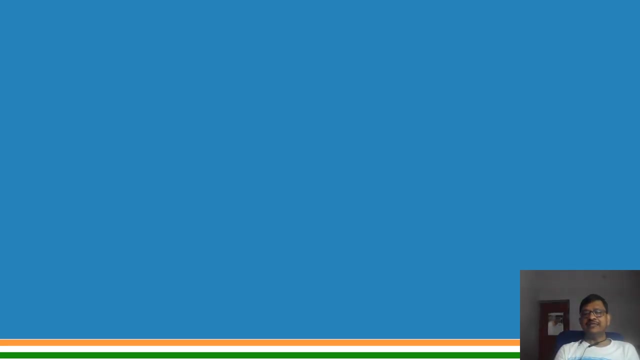 telecommunications. so with this, let me thank you for listening. so thank you. you can connect me on my gmail, which is ashokumar100 at gmailcom. please note that there is a single K in between: asukkumar. so there is a single K in between. so, finally, 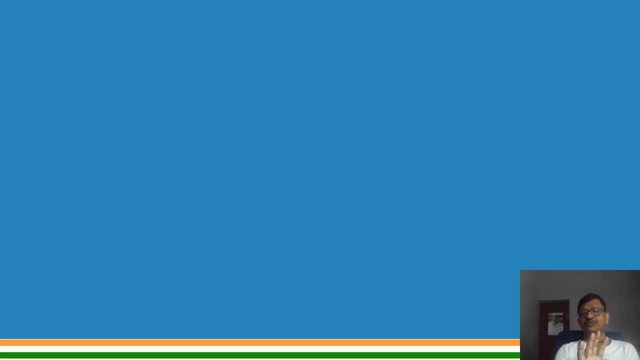 namaskar and bye for now. let's see you in the next video.